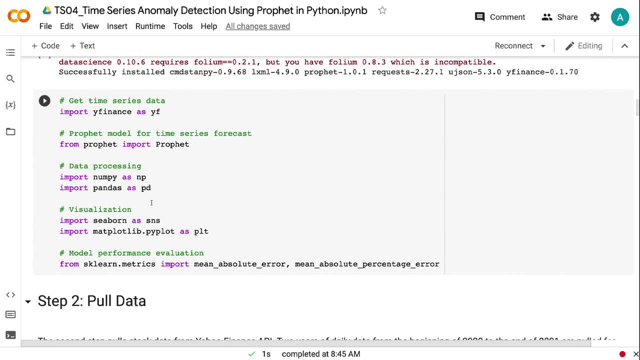 they are imported into the notebook. We also import pandas and numpy for data processing, Seaborn and mapletlib for visualization And mean absolute error and mean absolute percentage error for the model performance evaluation. To get the code for this tutorial, please check out my blog post on YouTube. If you have any questions, feel free to ask them in the description of this video. If you have any questions, feel free to ask them in the description of this video. Please check out my blog post on YouTube. If you have any questions, feel free to ask them in the description of this video. If you have any questions, feel free to ask them in the description of this video. 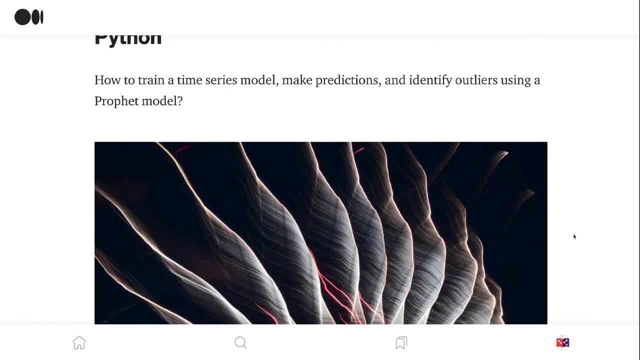 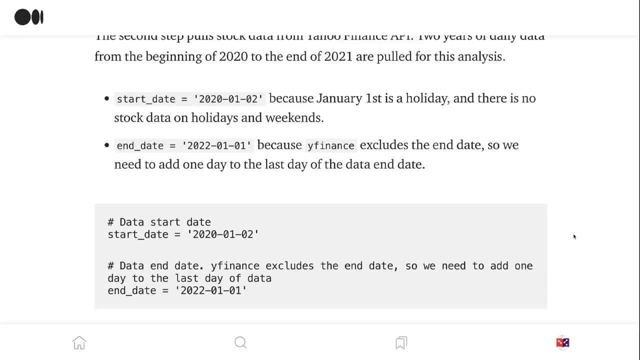 I will put the link in the video description. Mediumcom is my most referenced website for data science and machine learning. It charges five dollars per month for full access. I have been a mediumcom member for many years and that's the best five dollars I spent every month, If you. 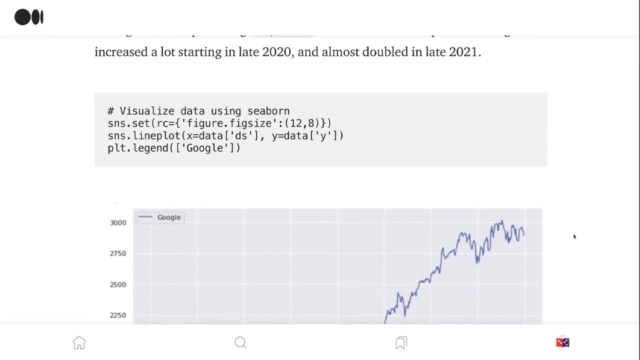 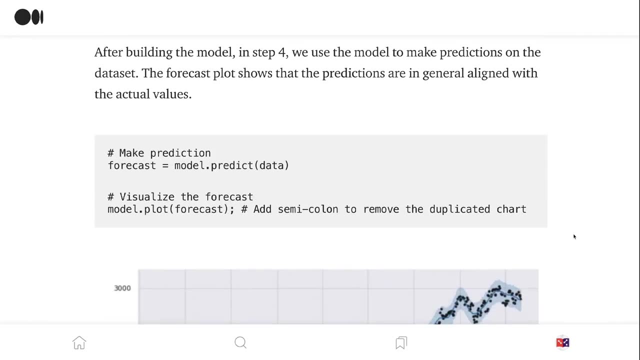 would like to support me and buy me a cup of coffee. please use the link in the video description to join the medium membership at no additional cost. If you prefer not to join, you can still read the post, because there are a couple of free posts each month for everyone to. 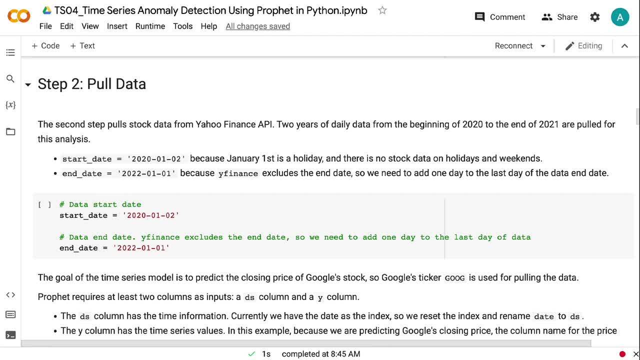 to read. Okay, let's continue with the tutorial. The second step pulls stock data from Yahoo Finance API. Two years of daily data from the beginning of 2020 to the end of 2021 are pulled for this analysis. Start date equals 2020-01-02, because January 1st is a holiday And there is no stock. 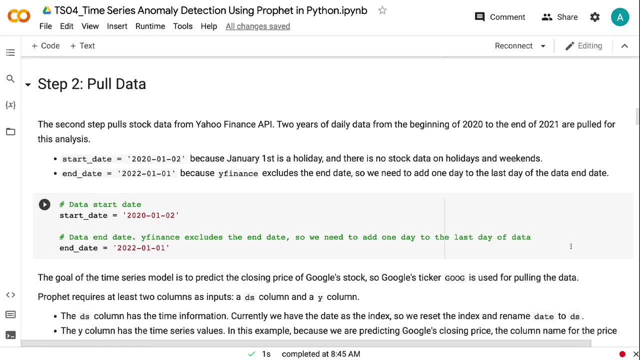 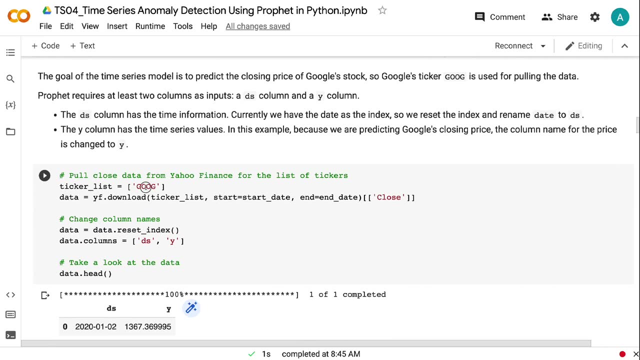 data on holidays and weekends End date equals 2022-01-01 because if finance excludes the end date, So we need to add one day to the last day of the data end date. The goal of the time series model is to predict the closing price of Google's stock, So Google's ticker GOOG is used for pulling. 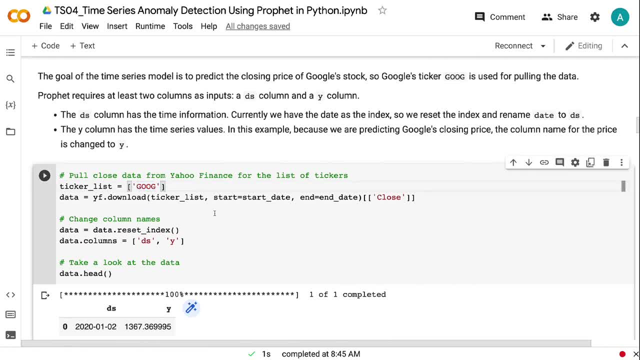 the data Profit requires at least two columns as inputs: A DS column and a Y column. The DS column has the time information. Currently we have the date as the index, So we reset the index and rename date to DS. The Y column has the time series values In this example, because we are 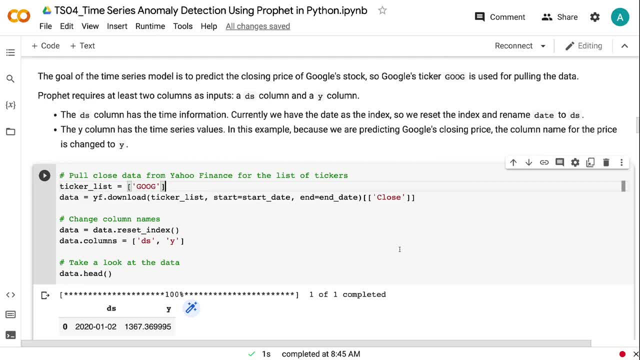 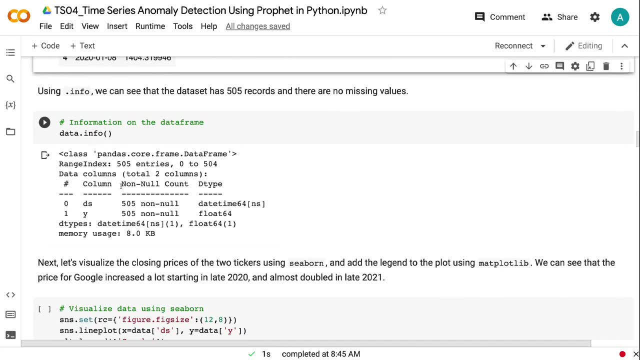 predicting Google's closing date, we need to add one day to the last day of the data end date. The column name for the price is changed to Y. using info, We can see that the dataset has 505 records and there are no missing values. Next let's visualize the closing prices of: 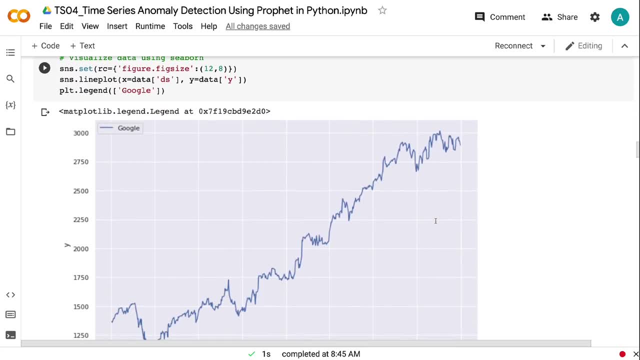 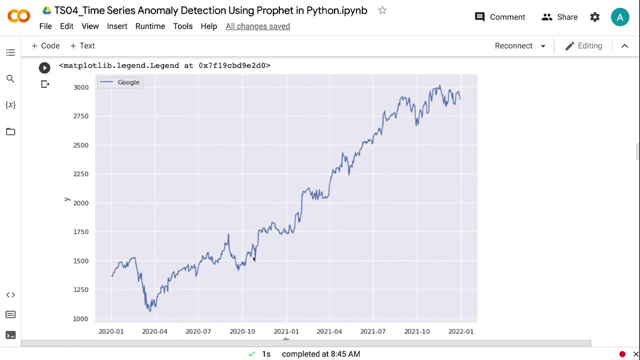 the two tickers using Seaborn And add the legend to the plot using matplitlib, We can see that the price for Google increased a lot starting in late 2020.. And almost doubled in late 2021.. And step 3.. We will build a time series model using Profit and Python. 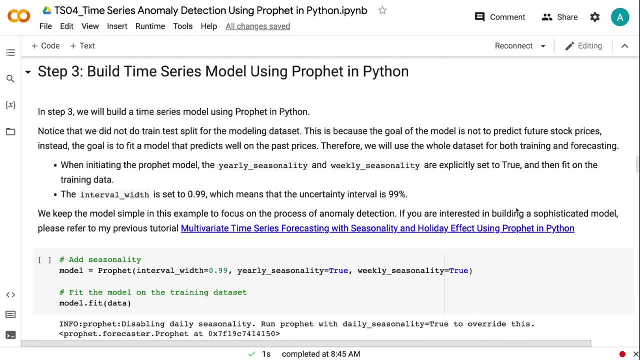 Notice that we did not do train test split for the modeling dataset. This is because the goal of the model is not to predict future stock prices. Instead, the goal is to fit a model that predicts well on the past prices. Therefore, we will use the whole dataset for both training. 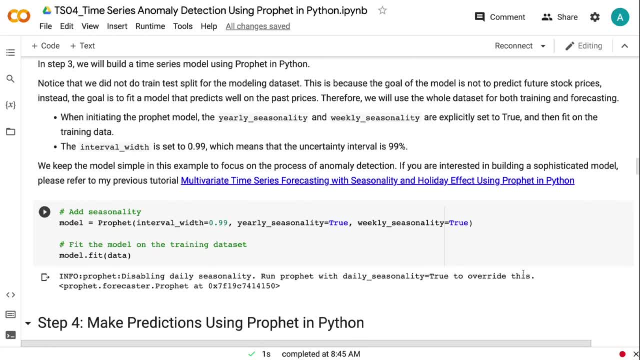 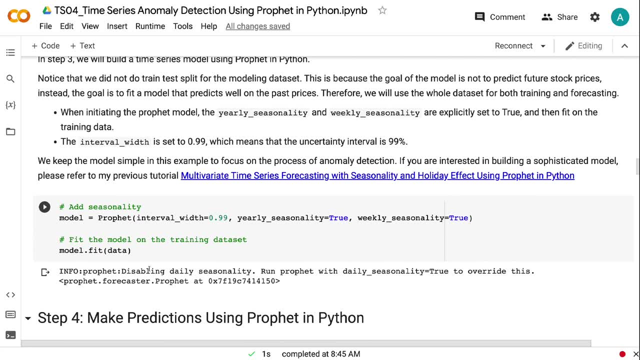 and forecasting. When initiating the Profit model, the yearly seasonality and weekly seasonality are explicitly set to true And then fit on the training data. The interval width is set to 0.99, which means that the uncertainty is set to 0.99.. And the interval width is set to 0.99.. 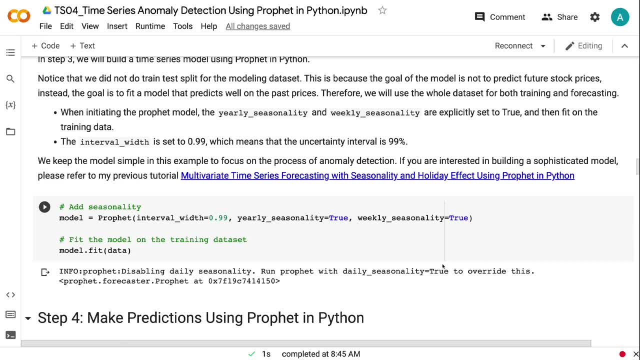 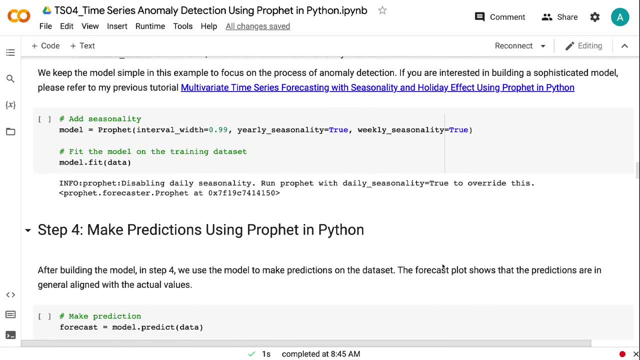 Interval is 99%. We keep the model simple in this example to focus on the process of anomaly detection. If you are interested in building a sophisticated model, please refer to my previous tutorial. Multivariate Time Series Forecasting with Seasonality and Holiday Effect using Profit and. 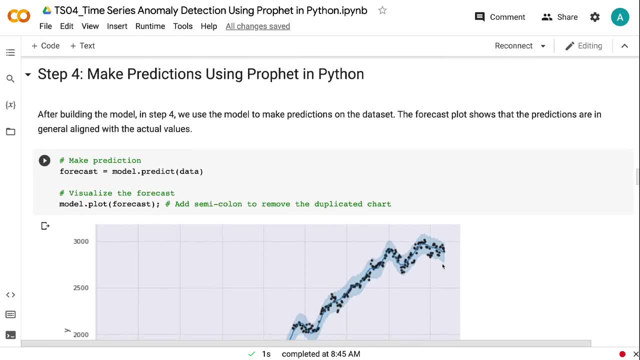 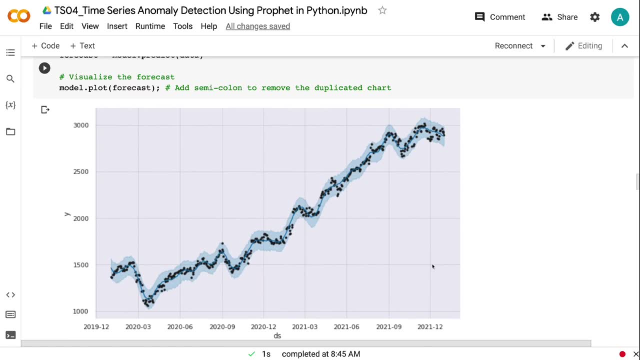 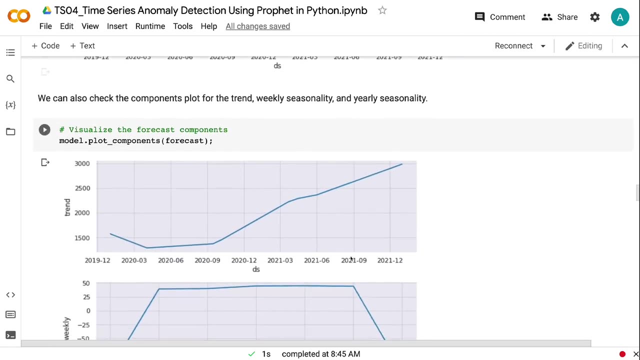 Python. After building the model. in step 4, we use the model to make predictions on the dataset. The forecast plot shows that the predictions are, in general, aligned with the actual values. We can also check the components plot for the trend, weekly seasonality and yearly seasonality. In step 5, we will check the time series model. 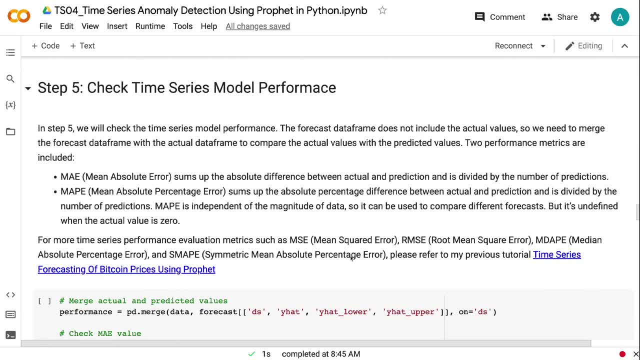 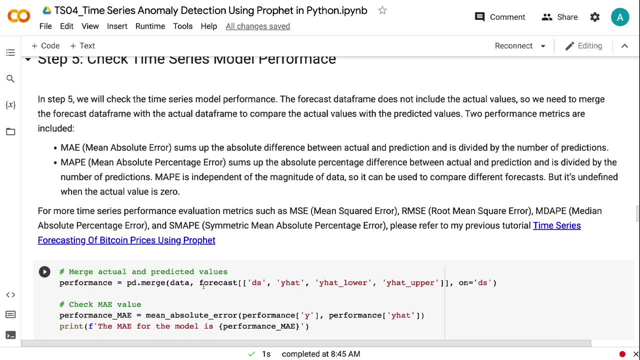 performance. The forecast data frame does not include the actual values, So we need to merge the forecast data frame with the actual data frame to compare the actual values with the predicted values. Two performance metrics are included. Mean absolute error sums up the absolute difference. 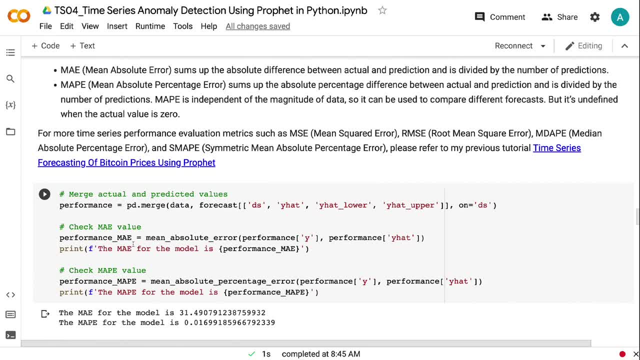 between actual and prediction and is divided by the number of predictions. Mean absolute percentage error sums up the absolute percentage difference between actual and prediction. Mean absolute percentage error sums up the absolute percentage difference between actual and prediction and is divided by the number of predictions. MAP is independent of the magnitude of data, So it can be.